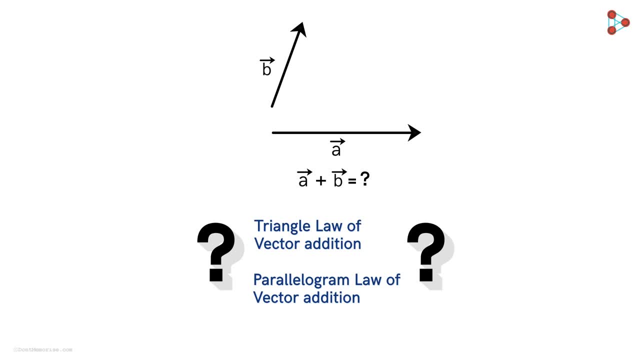 But which one should we apply here? Also, what if we want to find the difference between these vectors? How can we find this? Let's understand these things in this video To find the sum of vectors. it doesn't matter which of these two laws we apply. 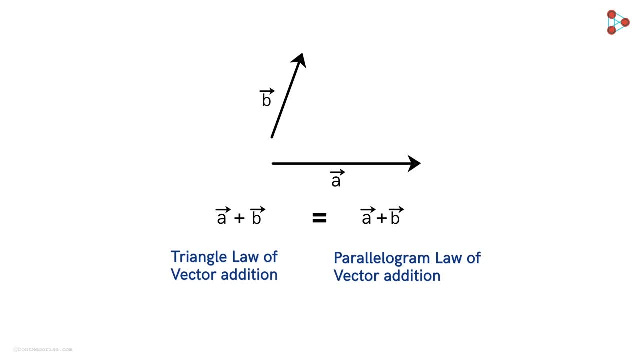 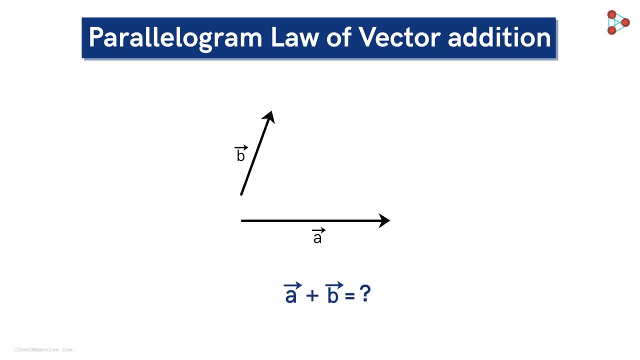 We will always get the same resultant vector. Let us see how. Let's first consider the parallelogram law of vector addition to find this vector sum. To apply this law, we move the vector B parallel to its position, such that its initial point coincides with. 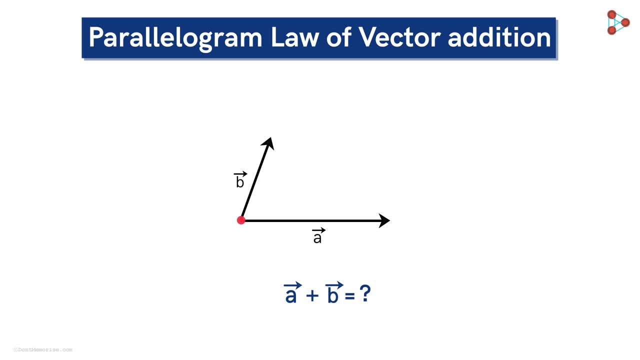 the initial point of the vector A, Then draw two lines parallel to the vectors A and B to form a parallelogram OACB like this. Now, this diagonal OC in this direction represents the sum of vectors A and B. We can also write this vector sum as this: 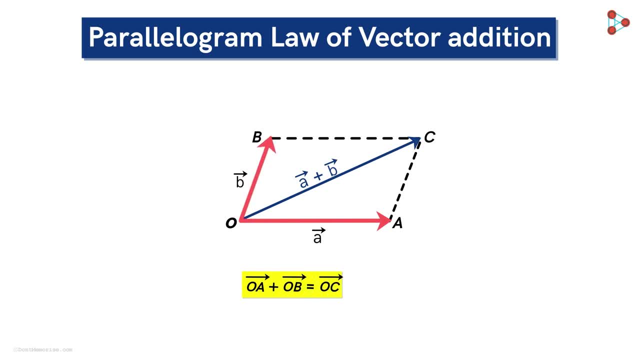 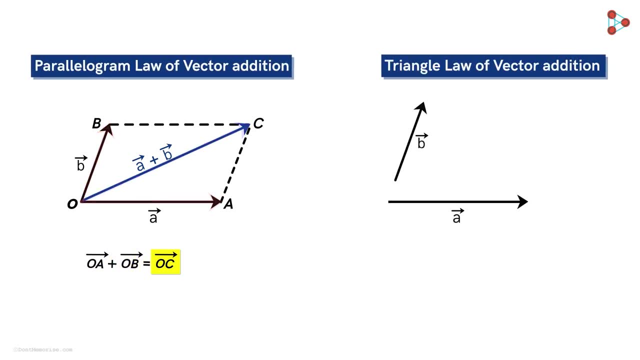 Vector OA plus vector OB. Vector OB is equal to Vector OC. Now let us see if we get the same Vector OC by applying the triangle law of vector addition. We know that to apply this law we have to place the vector B such that its initial point coincides with the terminal. 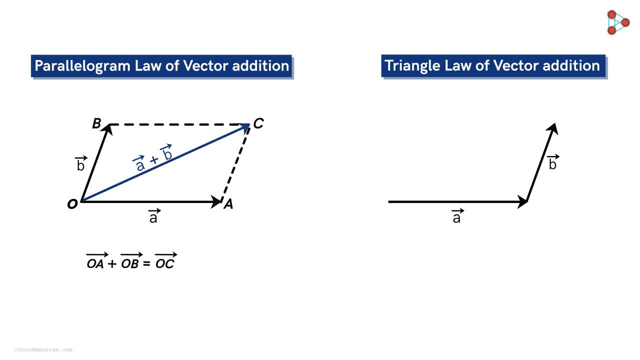 point of the vector A. Now observe this parallelogram. Notice that the side AC will be parallel to the vector B. And since this vector is parallel to the vector B, And since the length of the sides OB and AC will be equal, 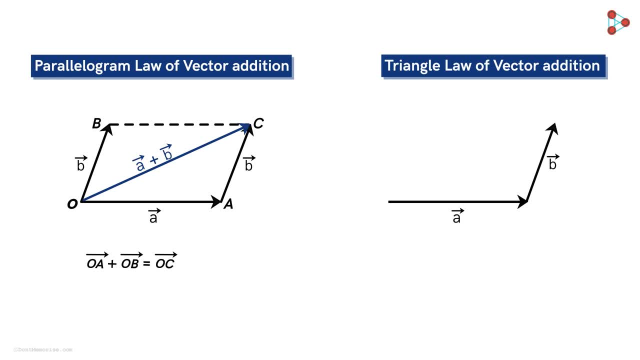 the vector AC will also represent the vector B. Now consider this triangle OAC. These two sides represent vector A and vector B. So according to the triangle law of vector addition, this side OC in this direction represents the sum of vectors A and B. 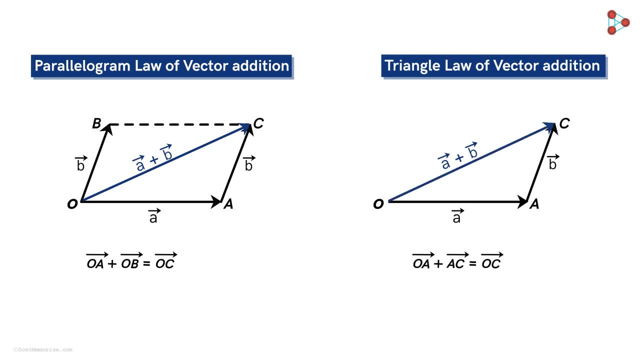 We can write it as this. Thus we see that by applying either of the laws, we get the same resultant vector as the sum of the vectors A and B. We can say that these two laws are equivalent to each other, That is, to find the sum of the two vectors. 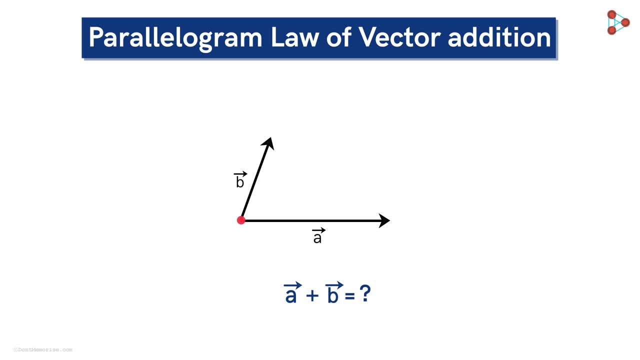 the initial point of the vector A, Then draw two lines parallel to the vectors A and B to form a parallelogram OACB like this. Now, this diagonal OC in this direction represents the sum of vectors A and B. We can also write this vector sum as this: 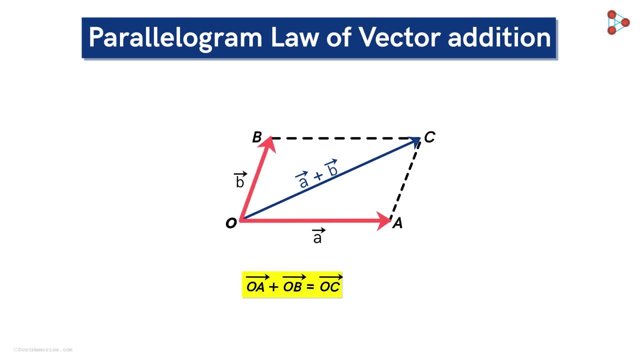 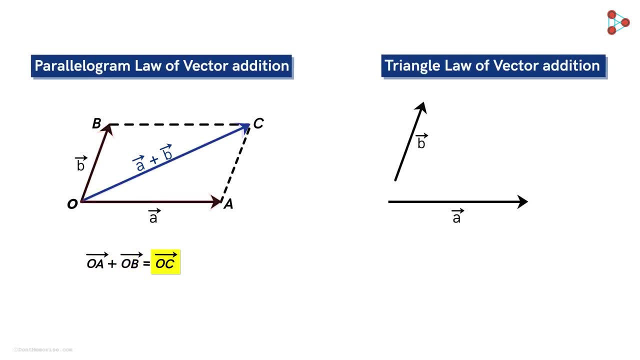 Vector OA plus vector OB. Vector OB is equal to Vector OC. Now let's see if we get the same vector OC by applying the triangle law of vector addition. We know that to apply this law we have to place the vector B such that its initial point 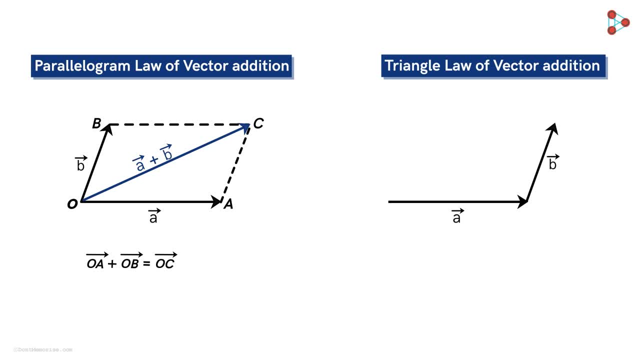 coincides with the terminal point of the vector A. Now observe this parallelogram. Notice that the side AC will be parallel to the vector B And since the length of the sides OB and AC will be equal, the vector AC will also represent the vector B. 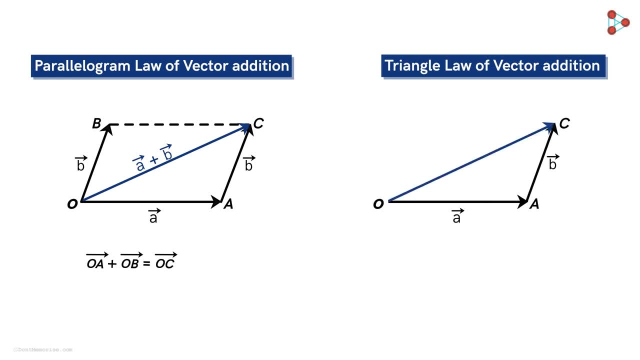 Now consider this triangle OAC. These two sides represent vector A and vector B. So according to the triangle law of vector addition, this side OC in this direction represents the sum of vectors A and B. We can write it as this: 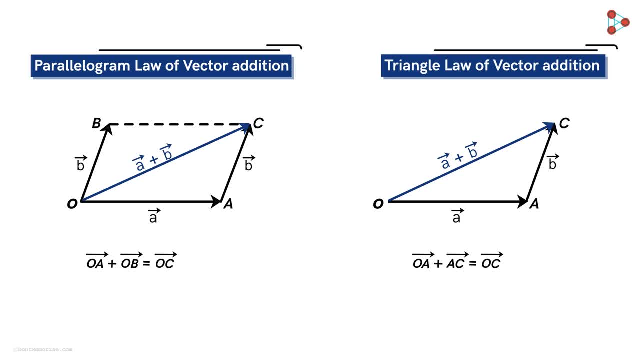 Thus we see that by applying either of the laws we get the same resultant vector as the sum of the vectors A and B. We can say that these two laws are equivalent to each other, That is, to find the sum of the two vectors. 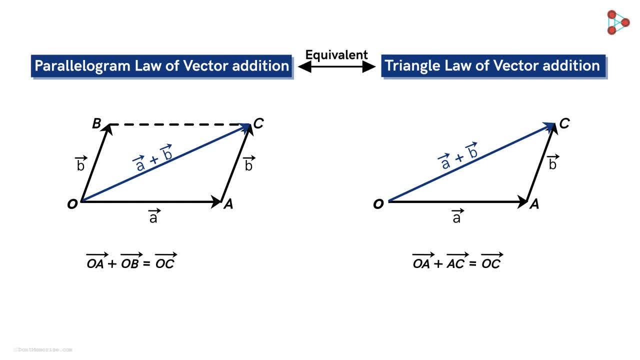 we can use any of these two laws. Now what about the subtraction of the two vectors? What does it even mean to find the difference between the two vectors? Let's find out Now. can you tell me what is 5 minus 2?? 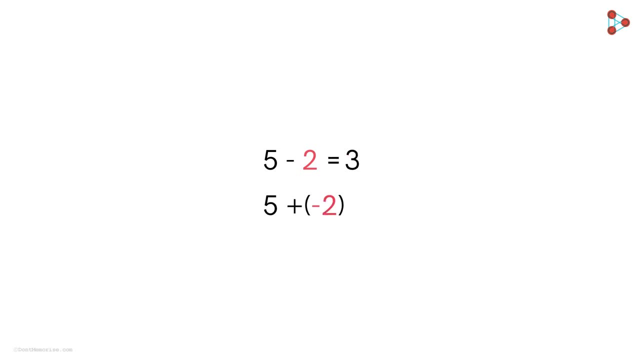 Right, It's 3!. And what is 5 plus negative 2? Right again, We know that even that is equal to 3.. So we see that the difference between two numbers can be written as the sum of the two numbers.